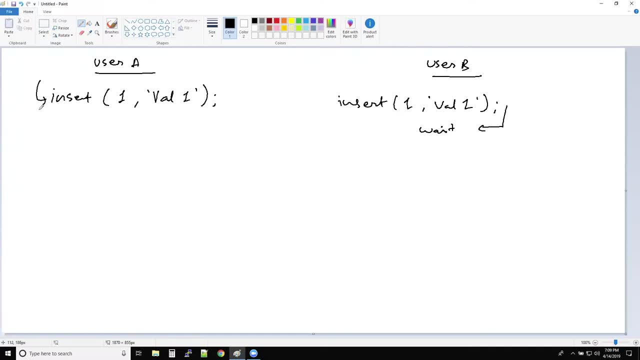 the user A is holding the lock for the record one and user B does not know what has to be done. And guys, this is the exact case with insert, update or delete, All right. So of course, we have already seen the example of insert. 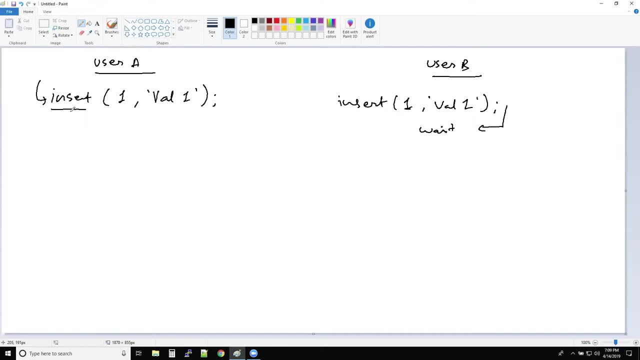 Let me get into an example of update for deadlock so that it will make more sense. You will get a variety in the example. Let us assume we have the test table. OK, Test table. and test table is having ID number. This is a primary. 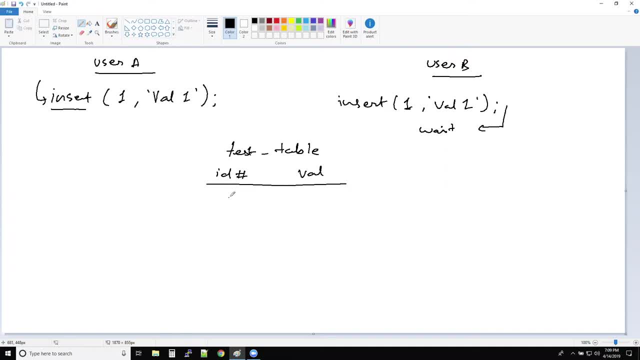 key and this is the value column. All right, So ID number is one, value is val1.. ID number is two, val2 and all right. We have multiple rows, but we'll stick to these two records. Now, assume that user A issued a command. 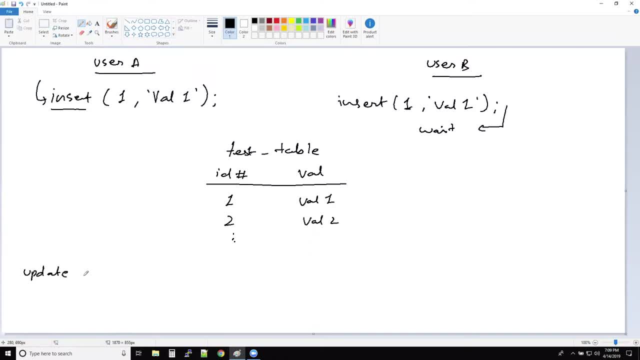 like update, update. val equal to guys. I'm not writing the exact SQL, I'm just trying to keep it simple: val equal to one, one, one, one where ID equal to one. All right, This is being executed by user A. Now user B is executing this. 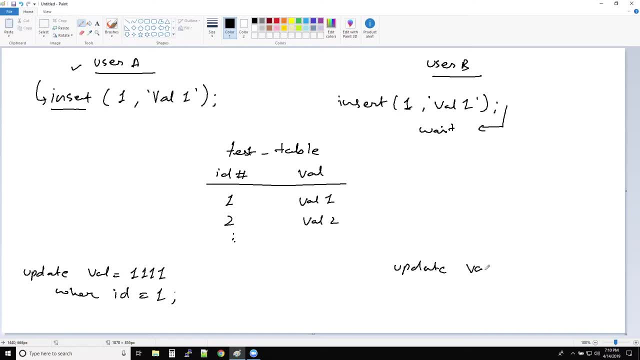 command update: val equal to double two. double two where ID number is equal to two, Right? So if you look at these records, OK, I'll create a column lock owner. So who is the user who is owning the locks for the records? for record one, the user. 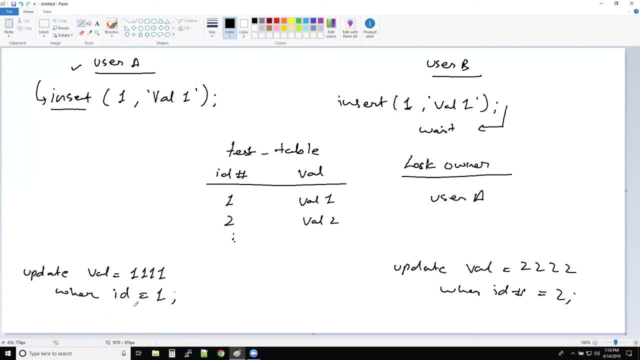 A holds the lock because over here you can see, the ID number is one, So the record where ID number is one, This will be locked and the lock owner will be user A. because user A issued this command for record to the user B will be the. 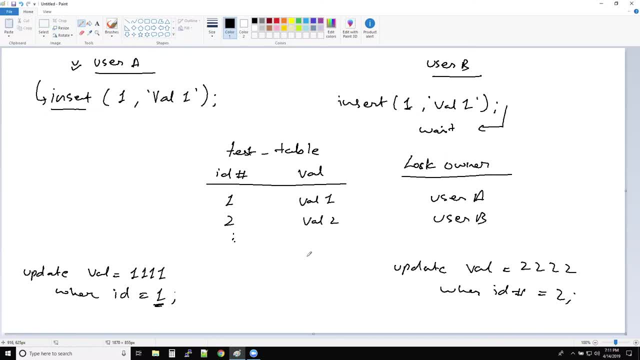 lock owner right over. here We are going with row level locks because both the users are trying to update different records at this stage. Assume that user A now wants to update the record to, because user A doesn't know somebody holds the lock for this record, So what user A will issue? 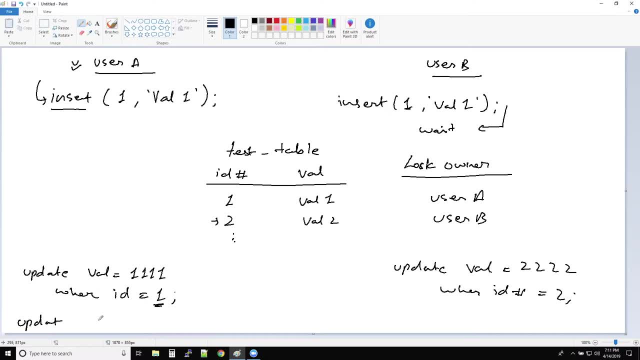 user A is trying to issue update val equal to double two. double two where ID equal to two. Now, once the user hit enters, what will happen? Can anyone tell me the answer? Guys, none of the users committed or rolled back the data, So don't get that in between. 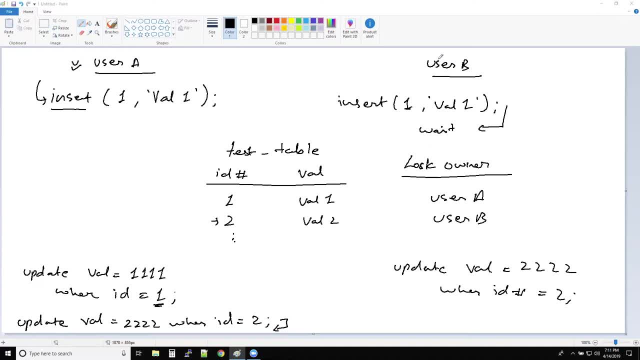 So what will happen at this stage? Hello, It's going to throw an error. It will not be able to insert, He will not be able to, He wouldn't be able to update. But why? Because user B has not done any commits, or. 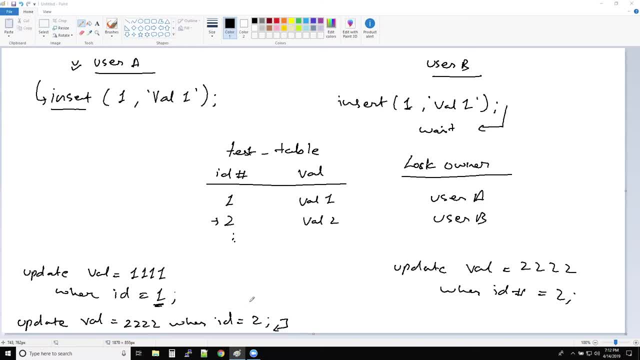 roll over. Okay, He's going to wait. A will be waiting. Right, It will wait for user B to either to commit or roll back. only then the user A- that val equal to two- will get updated or Correct. That's right. 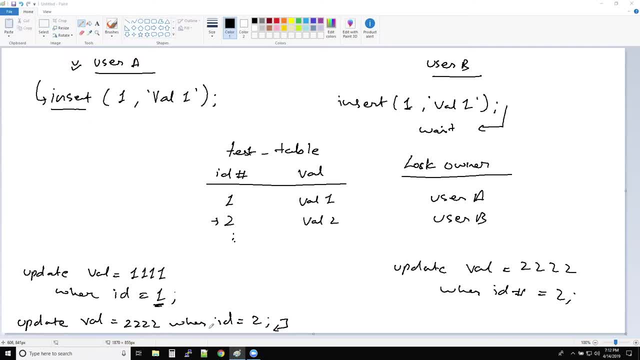 That's right, guys. So the thing is like: over here, Akechi, see this command. It's very simple. Whenever you are confused, the thing is like you have to understand if somebody is already working. We see that user B is working on ID number two, Right? So 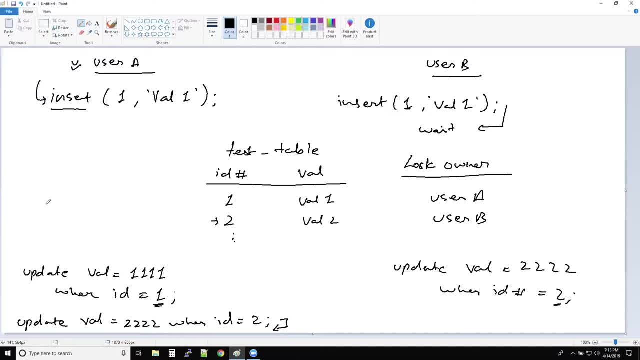 with. I don't know why people get confused, but you need to be very clear. Did the user commit or roll back? It's very simple, Only three conditions. Did the user roll back, Did the user commit or did the user disconnect from the database? 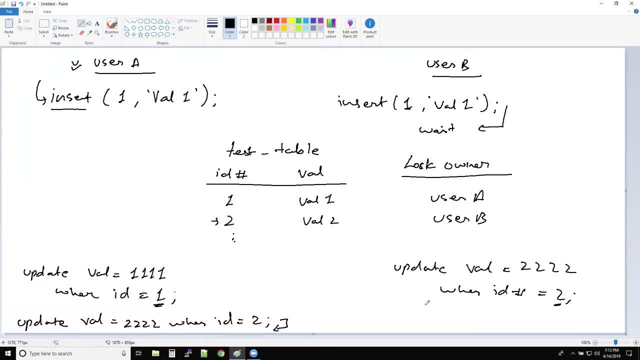 These are the only three scenarios where the locks will be released, So you don't have to be confused. right now. The lock is hold by whom? the user B, correct? So user B holds the lock. User A is trying to update the record. What will happen? The user A has. 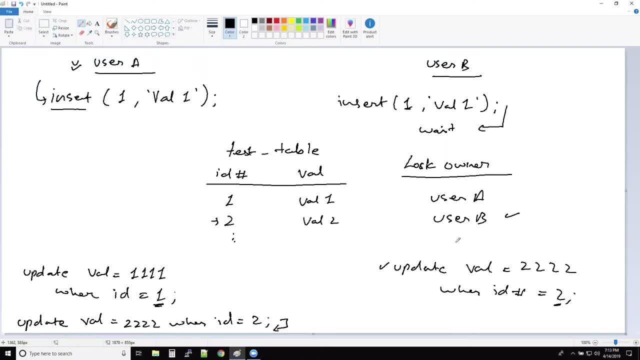 to wait because the user B needs to release the lock so that user A will get the lock. So in any insert, update, delete command, The first thing that happens is acquiring the lock. So the user who is working on the record will acquire the lock. In this case, 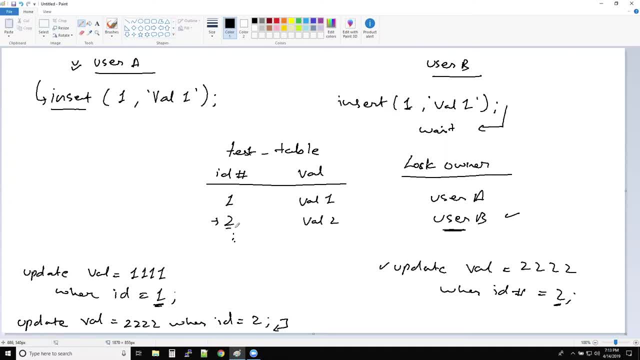 user B is already acquiring the lock on ID number two and the user A is trying to update the same record where ID is two. So user A has to wait until B commits rollbacks or disconnects from the database. Now, in this situation, what is happening is this session goes on wait. 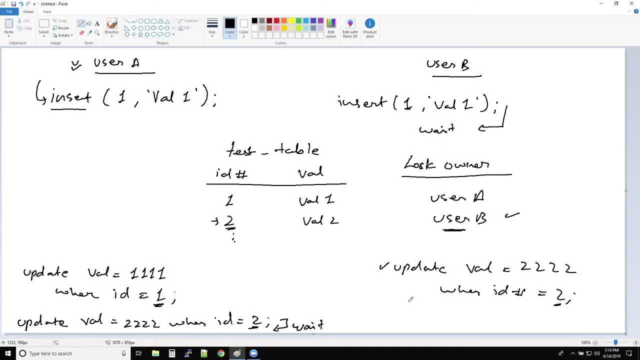 All right Over here, the session B. the user B now believes that I mean the user B wants to update the record one. So update, Well, sorry, Well, equal to one, one, one one where ID equal to one. Now what will happen? Tell me, Come on, Ikechi At this. 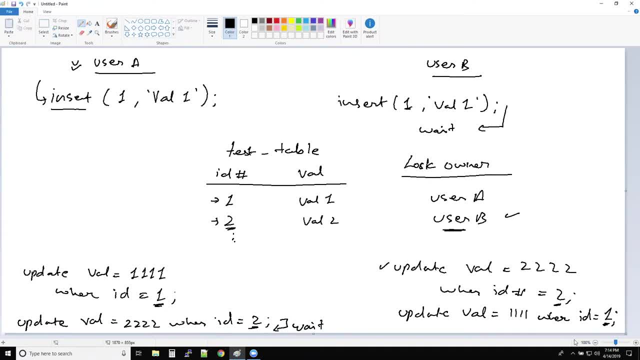 stage. Yes, if user A has not committed a rollback, the user, user B, is going to be on wait. So the user A is waiting for B to release the lock on record two. Okay, Now, if you say Yeah, It became a deadlock. now It is both trying to get. 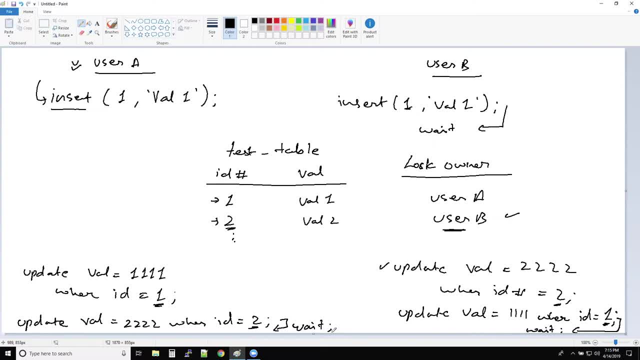 other lock Right. So in just for others to know, in this case what happens is both the sessions are waiting for each other to release the lock. User A is waiting for B to release the lock on record two and user B is waiting for user A to release the lock. 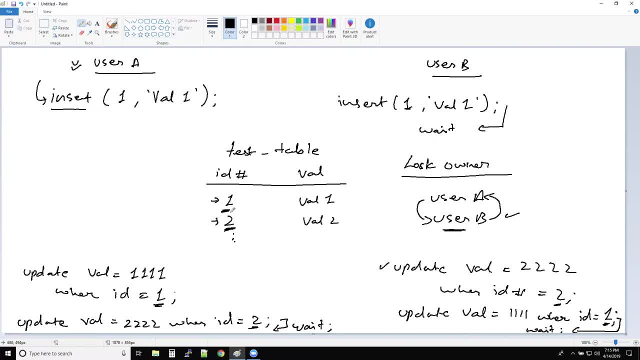 on record one, And this will continue infinitely. Now this is a big problem inside the database and this situation where one user is waiting for the other user to release the lock, when two or more sessions are waiting for each other to release the locks, The 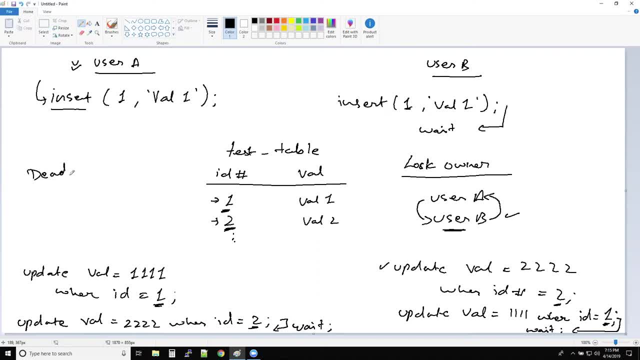 situation in is known as deadlock. Now the question is: what do you have to do in a deadlock situation as a DB? First thing: you do nothing because Oracle is smart enough and Oracle can detect deadlock within three seconds. All right, So for the user B, when the 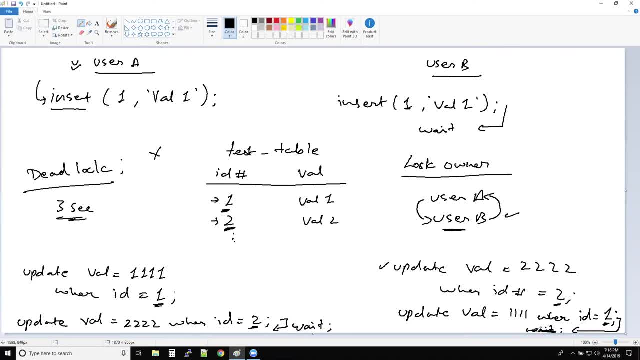 user B hits enter, the user session will not be waiting, rather Oracle will say deadlock. So Oracle will throw an error saying like deadlock situation has occurred. But if Oracle is waiting for B to release the lock, what will happen to this session? because this command is still waiting for session B, right? So what will happen? 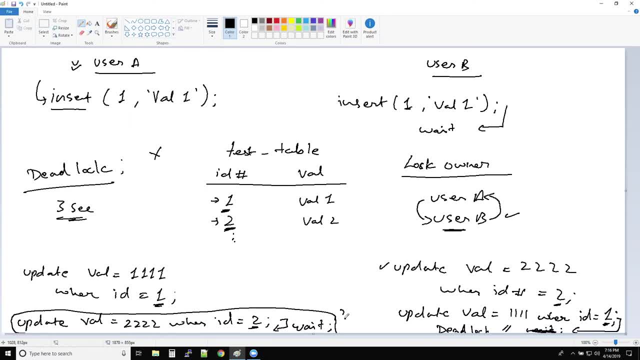 to this command Over here. the Oracle gave an error: right deadlock detected. Okay, this command is ignored. But what will happen to this command? Does I mean our Oracle will give the lock to the user A or what will happen? That will be completed? Any other guesses That will? 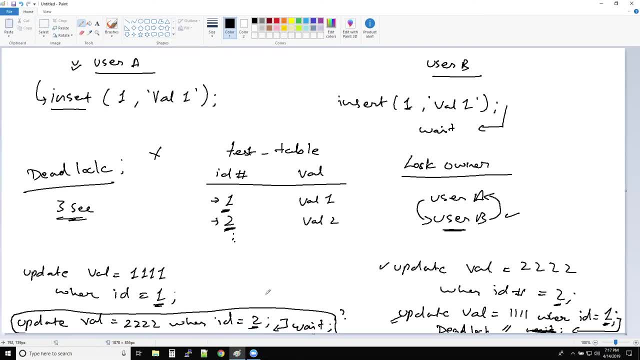 still continue waiting. Right, See, guys, this command what it needs. it needs user B to commit, rollback or disconnect, right, But nothing of that sort happened in the session B. Session B gave an error for an update command because there was a deadlock situation, But this: 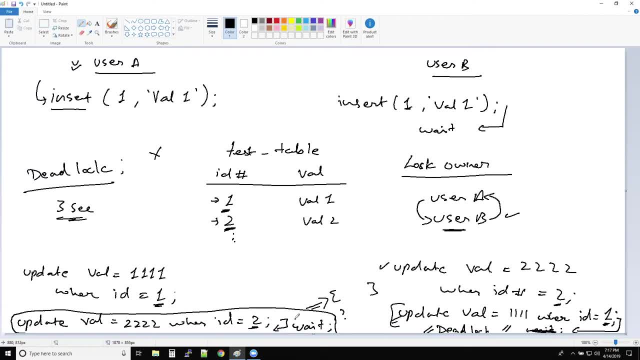 command from user one will continue to wait because user B still did not commit or rollback. Now what I mean? I think I would suggest you guys. I can show you an example, But I think this is a very simple example. I want you guys. 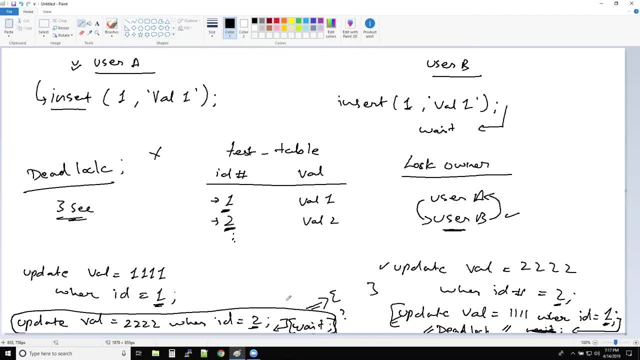 to create this scenario in your system. It is very simple. first try to update a record like this, then run in the second session, run this command So that each user is getting a lock on a different record and from the session one try to update the record where the 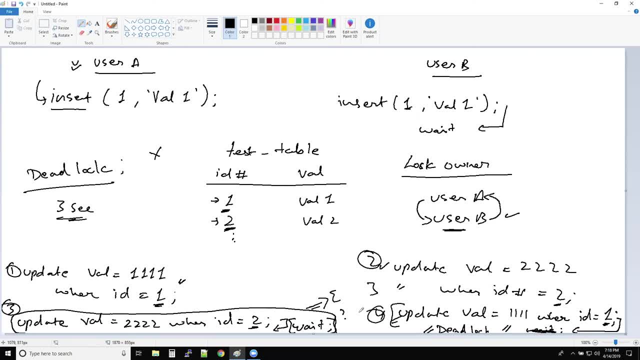 lock is hold by the other user, and then, same way, you execute another update which is trying to acquire the lock which was run in step one. So what you do is like create a test table exactly like this, just to understand how deadlocks work and what. 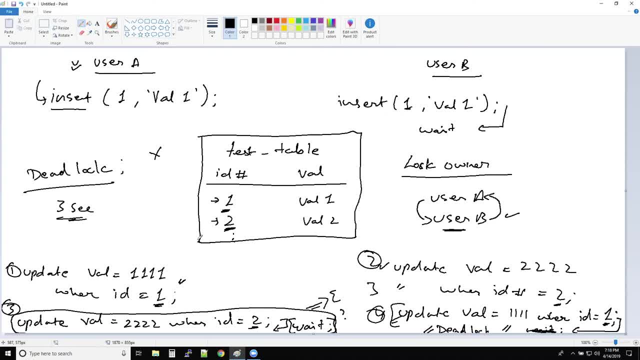 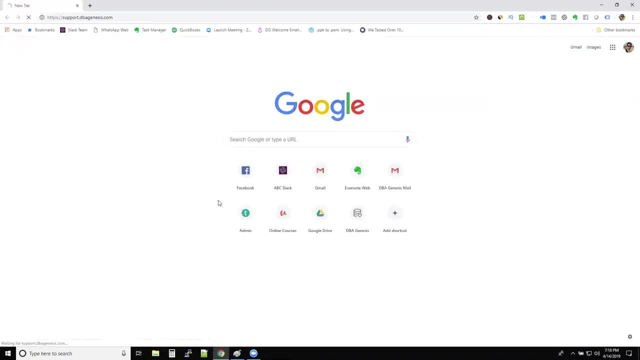 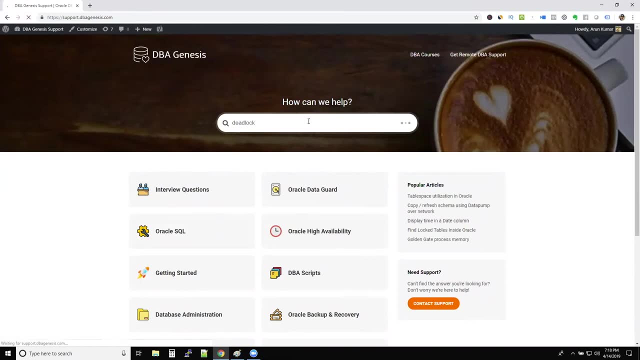 you do is just identify and work on the deadlocks. I think I also have a document with the same example, not document, I think, the article. I'll show you the article quickly and then and then locks. I think it is how to work with removing 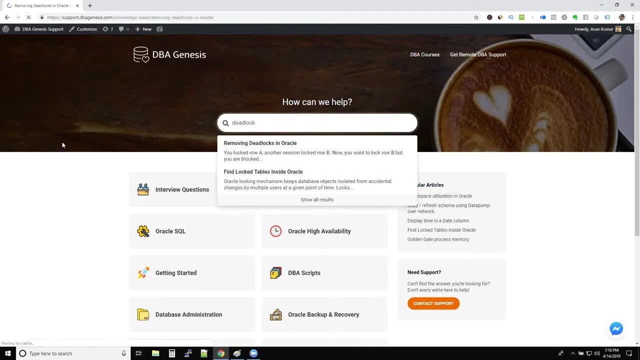 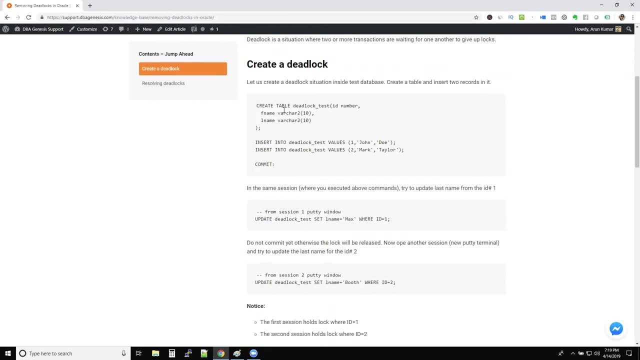 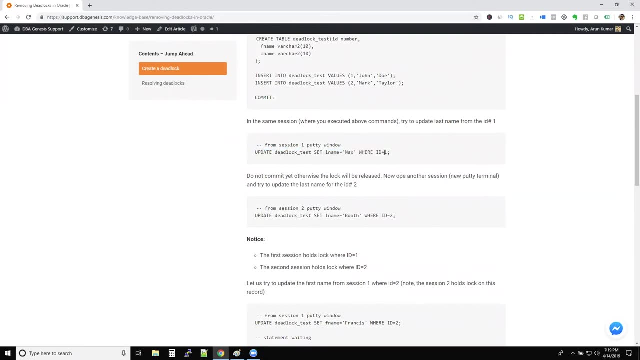 deadlocks in Oracle. So I give the same example like this: like there are two records We are inserting in a table, We are committing, and then we are opening a new session. We are updating the one record where ID is one We are updating in a. 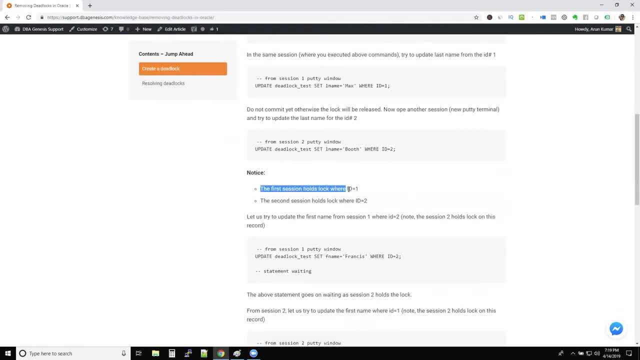 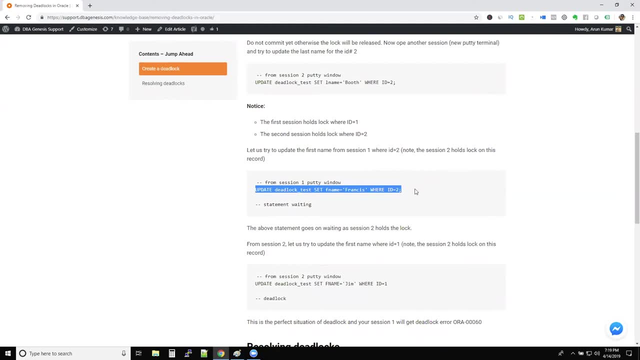 second session where ID is two. The first session holds lock on ID one. second session will hold lock on ID two and then you try to update from session one on session to record from session to session one and this will encounter a deadlock. You can see. 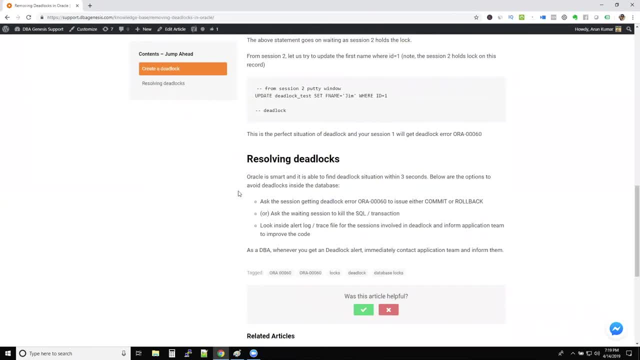 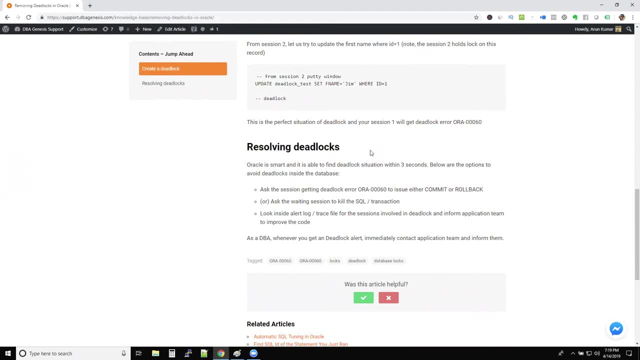 in first session statement Will be continue to waiting. So how do you resolve the deadlocks? This is important enough. First of all, deadlocks are very simple. whenever there is a deadlock, Oracle knows it and Oracle will detect it immediately and then throw an error saying like aura. 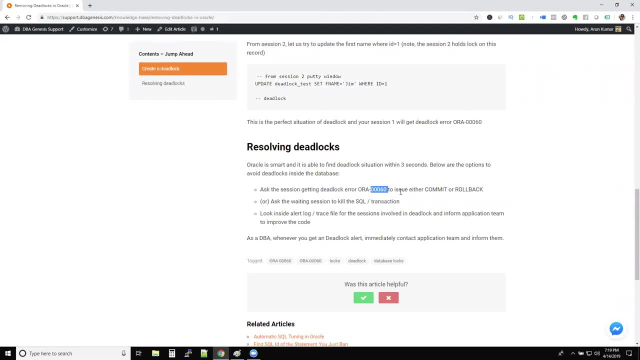 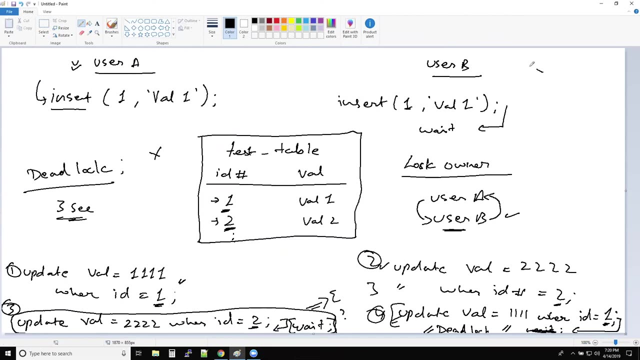 triple zero, six zero. So what you can do is ask the session getting deadlock error, like aura zero, six zero, to issue either commit or rollback. Now in this case, Now in this case, guys, If this user B is saying like hey, I'm getting deadlock error again, 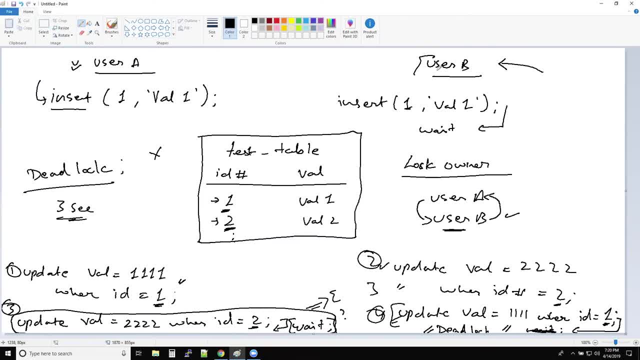 and again I'm trying to update a record. you ask the same user: Hey, can you actually issue a commit on a rollback? because the user B is getting deadlock error because the user is waiting for user B and user B is waiting for user a. so if the user B commits, 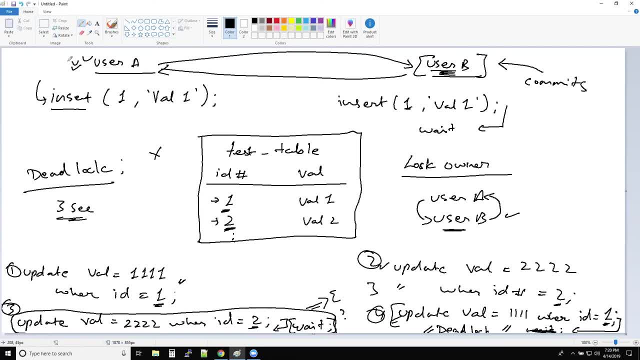 What happens is. What happens is user a will no longer wait for user B, and then you can ask the user behind. once you commit, you rerun your command and then it will execute. you ask the user be the person who's getting the deadlock error, to commit or rollback. 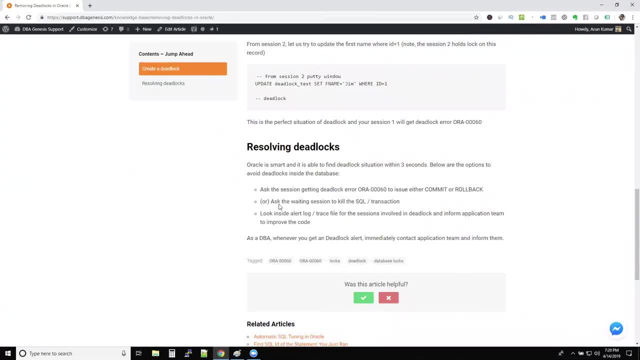 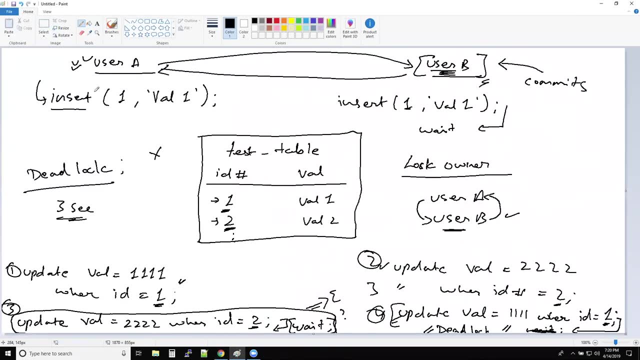 All right, so that's the first step. or you ask the waiting session to kill the SQL transaction. What you can see is: like the user a: This is the waiting session, right, The user is waiting over here. So you can ask user a like: hey, can you stop the SQL query, or can you? 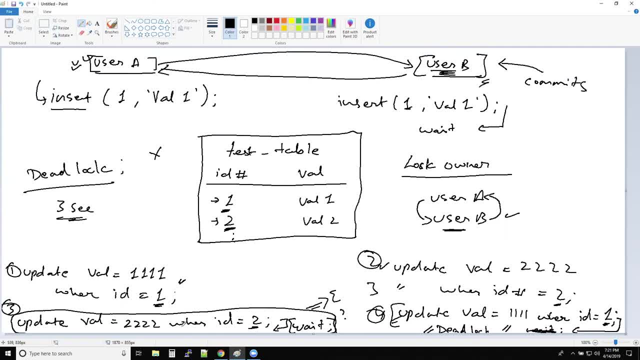 quit your SQL query. Maybe they can press control C, control X on their terminal. But sometimes these are not the queries that humans will run. These are run by the application, So that point of time it's hard for the waiting query to be quit. 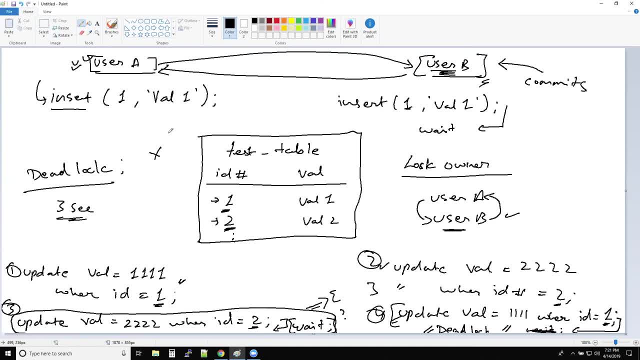 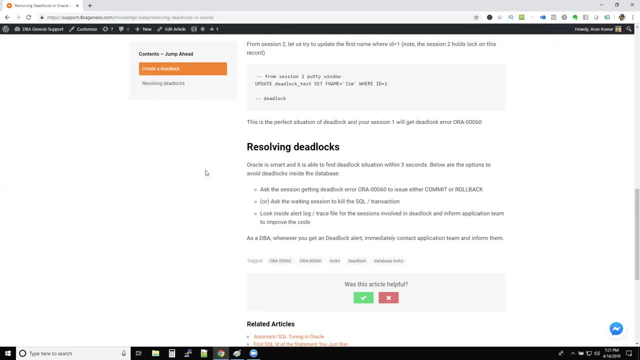 But in general I'm saying like in your scenario you can quit the user a and say that, hey, can you kill the SQL that you're running, And then what you can do is whenever there is a deadlock situation. The problem with deadlock is guys. 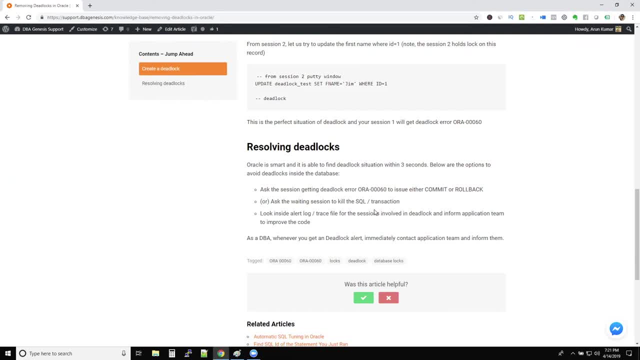 It occurs because of a poor design of application. So the application team, the design the application in a way where multiple queries Are trying to update, delete, insert, and then there is a lock conflict and because of which you might see a lot of deadlock errors or our. 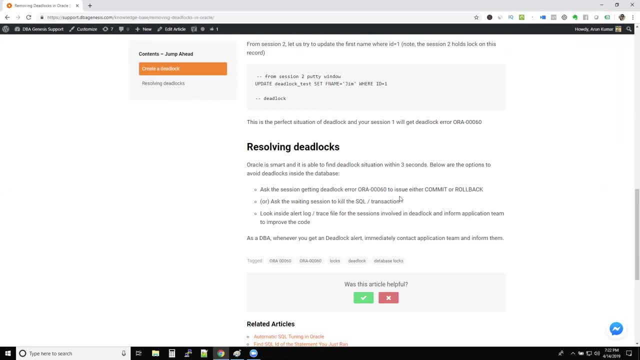 triple zero, six zero in the database alert log. So what do you do in this situation? Your job is, whenever you see this error, of course the solution I already gave you- ask the session which is getting deadlock error to commit or rollback. But your job as a DB should be to inform. 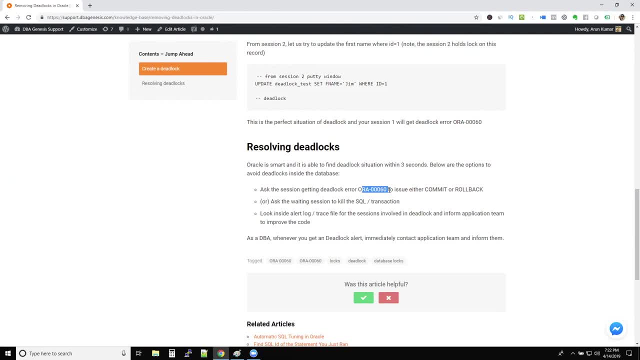 The application team. Hey, can you modify your code or your application so that there are frequent commits in case, if they are trying to insert a bulk load or something, or you ask them, can you kind of like make sure the sessions are not waiting for each other and then you kind of like give your own? 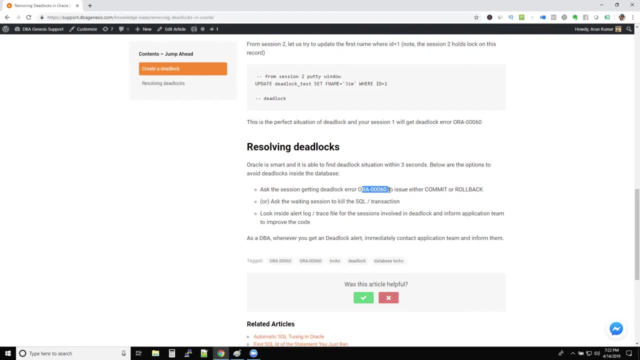 recommendation saying like: what are the situations when deadlocks occur? because sometimes the application team or the developers- Of course, nowadays all the developer developers are smart enough, but still sometimes you as a DB need to tell them what is deadlock when it occurs, so that they themselves can review their code and modify it.